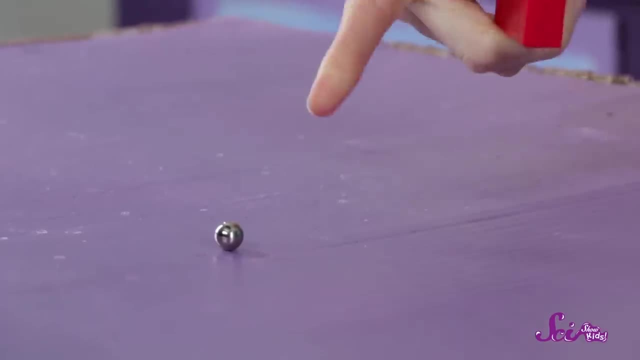 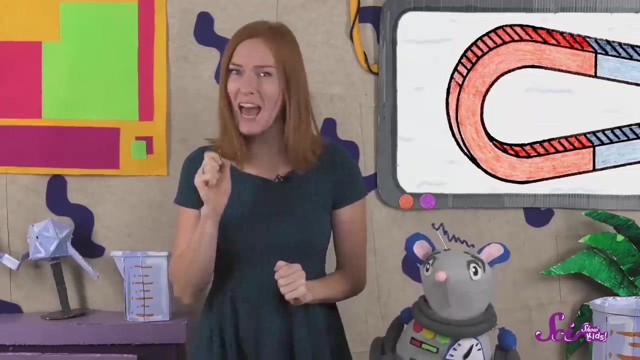 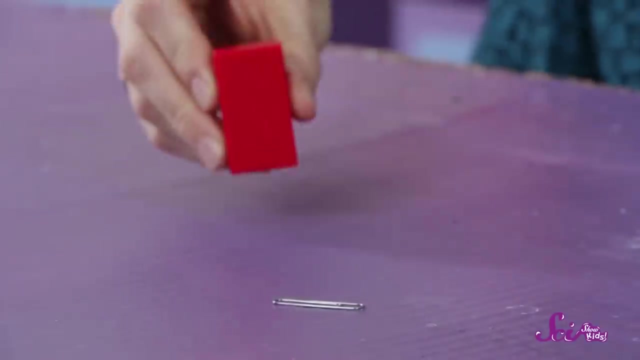 The magnets that are in my toy pull on or attract this little ball and when they get close enough they stick to each other. If you have a magnet at home, you can see how it attracts this kind of a paper clip. If I move the magnet slowly toward the paper clip, the magnet pulls on the paper clip. 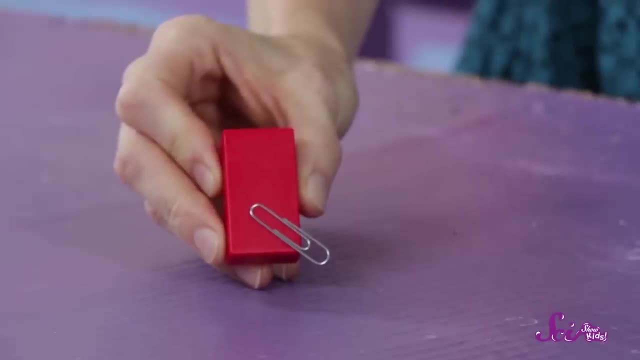 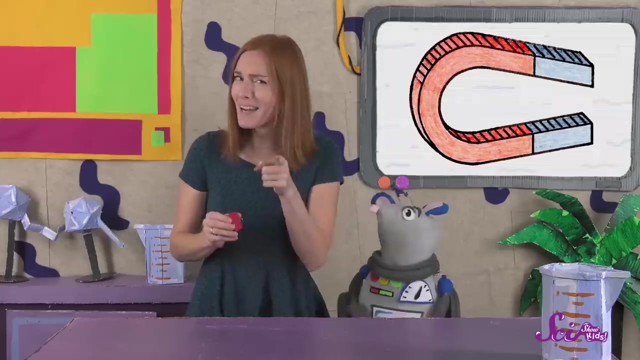 until the two objects are completely stuck together. And once they're stuck, they stay stuck until I put a force of my own on the paper clip by pulling them apart. You might have noticed that I didn't even have to touch the magnet to the paper clip. 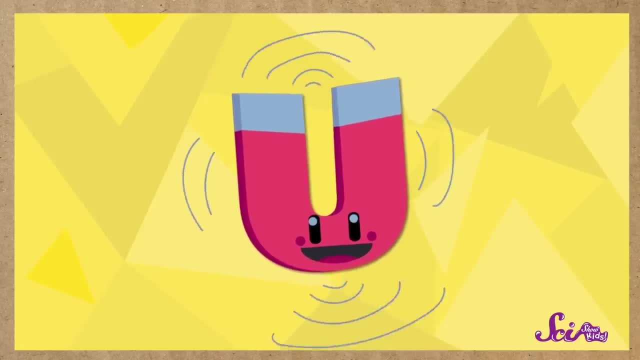 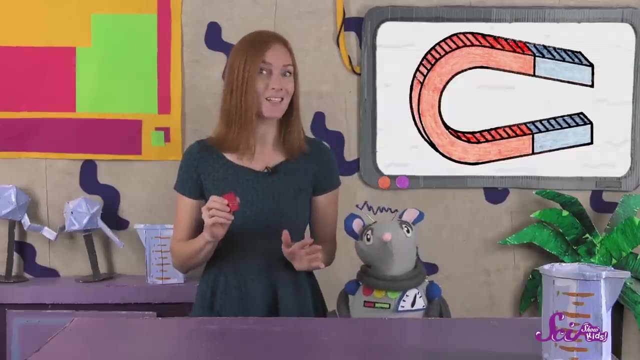 to get them to stick together. That's because there's an invisible area all around the magnet that can attract certain things called the magnetic field. You can see how strong a magnet is by seeing how close you have to get to the object before the magnet starts to pull. 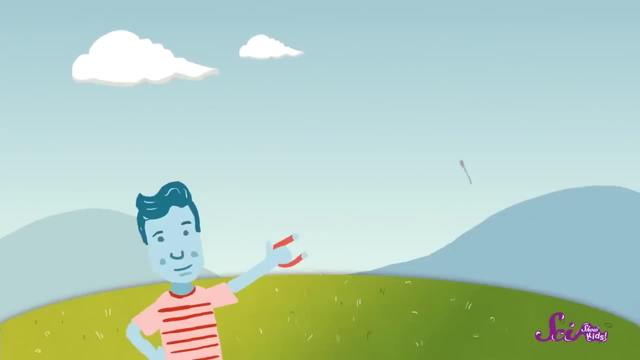 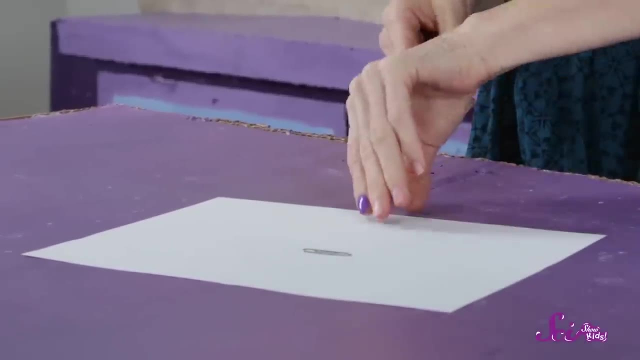 If your magnet is pretty strong, it'll be able to pull objects that are farther away than weaker magnets, And a magnetic field can do some pretty neat things. Check this out: If I put my paper clip on top of this paper and my magnet below the paper, I can move. 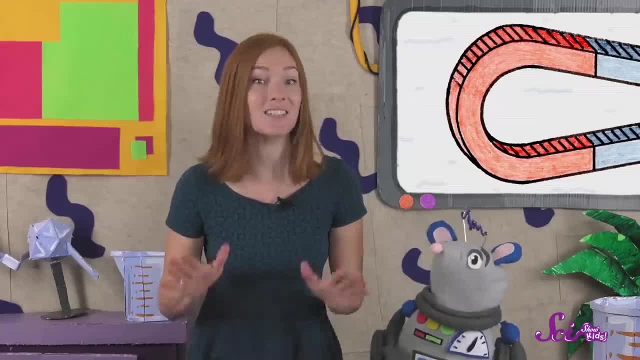 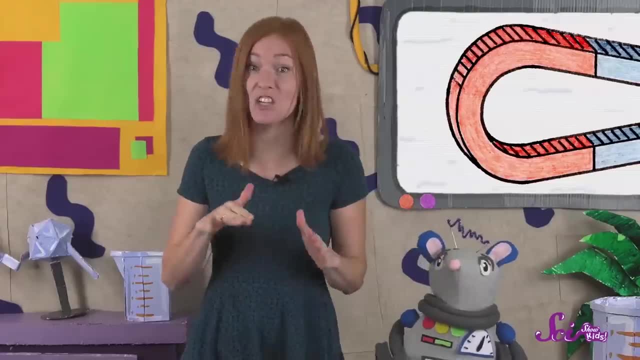 the paper clip without using my fingers at all. That's because the invisible magnetic field pulls on the paper clip right through the paper. Even though the magnet isn't actually touching the paper clip, it's still pulling on it, and that's enough to make the paper clip. 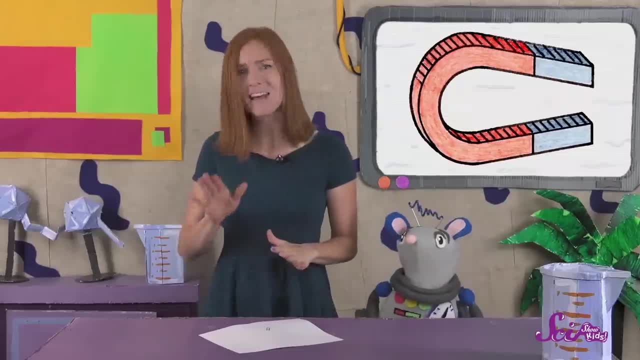 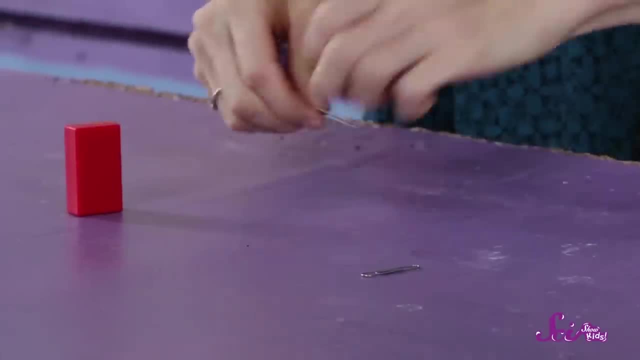 But just because something is attracted by a magnet, that doesn't mean it's a magnet itself. For example, we just saw that my magnet sticks to this paper clip, but the paper clip won't attract or stick to another paper clip. That's because it's the magnet that's special and doing the attracting. 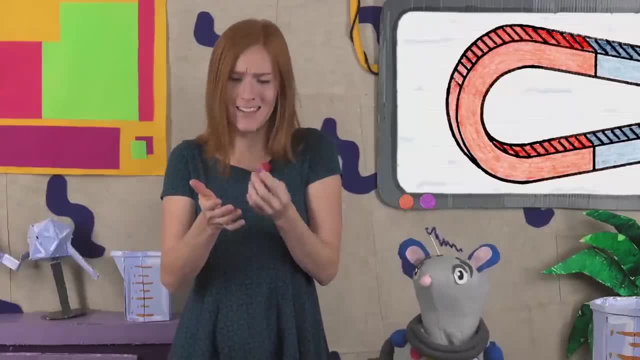 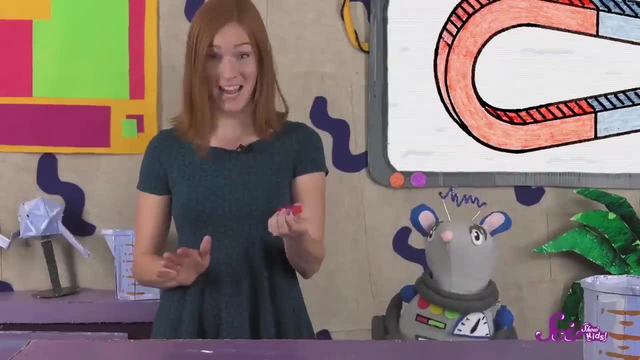 Now, magnets don't attract all things. For example, this magnet doesn't stick to me, but it does stick to Squeak's nose. The magnet also isn't attracted to the table, But we already know it attracts things. It attracts the paper clip. 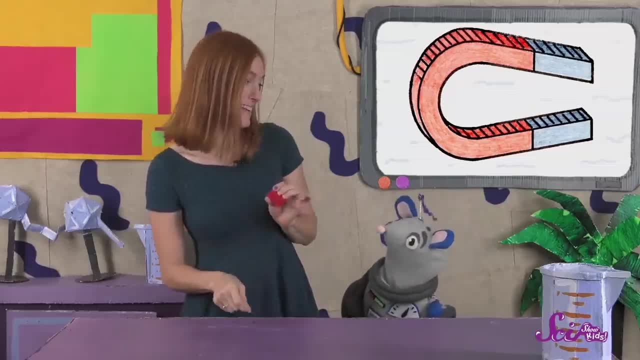 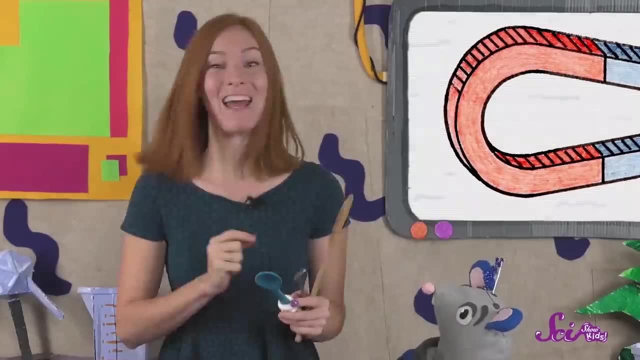 Hmm, I wonder what other things will stick to my magnet. Let's go find some stuff around the fort and do an experiment. OK, I have some spoons from the fort's kitchen. Let's play a game. I'll hold up a spoon and you and Squeaks can guess if the magnet will attract it, or 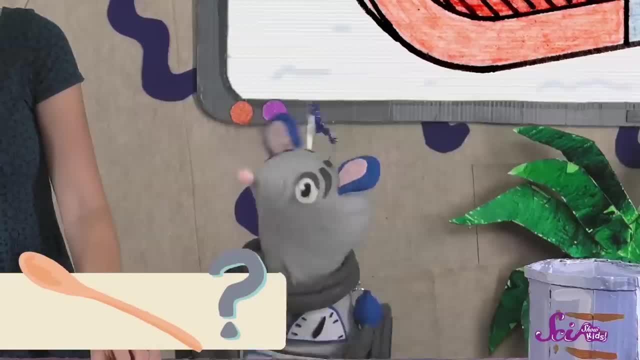 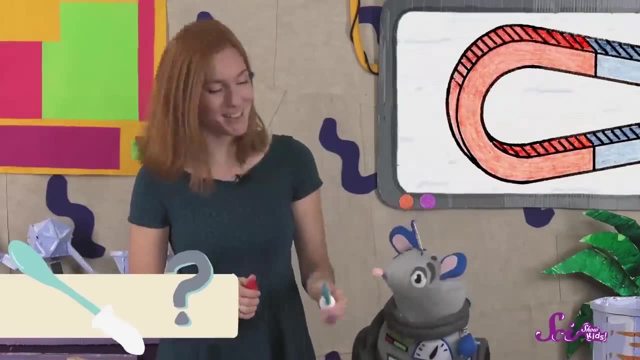 not. First, let's try this wooden spoon. What do you think Squeaks? Good guess, Let's try it. You're right, It doesn't attract the wood. OK, let's try this plastic spoon. What do you think Squeaks? 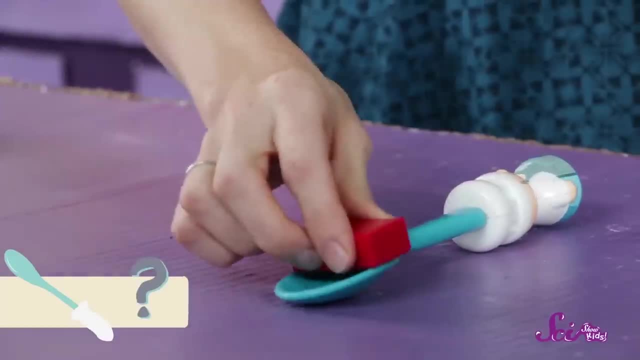 No, again, Let's try. You're right again. Magnets don't attract plastic. OK, let's try our last one. What do you think Is it going to stick? Alright, let's try. Ah, they do They stick. 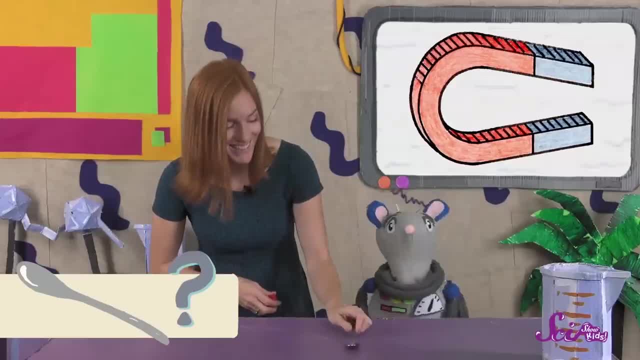 Look at that. So let's see, Of all the things we tried, the magnet was only attracted to Squeaks' face, the little tiny ball, the paper clip and this spoon, And there's something they all have in common. 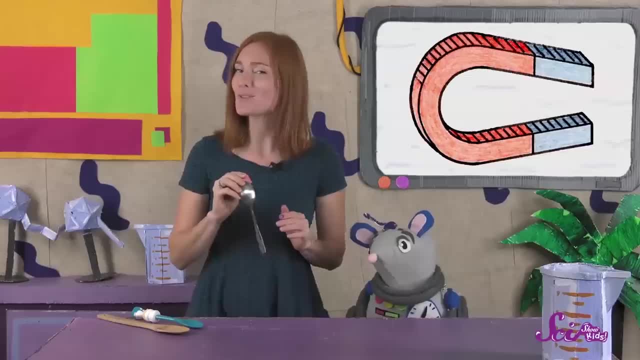 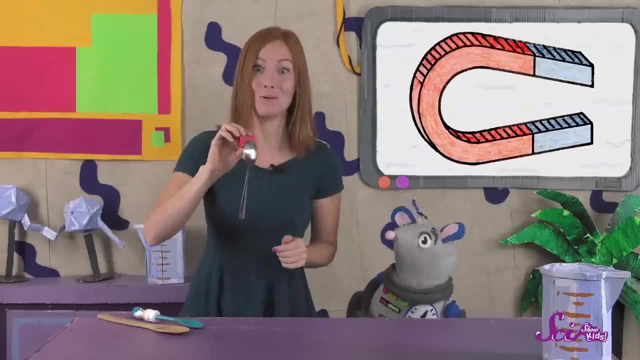 It's the same thing, It's the same thing, It's still the same thing. It's the same thing, Then, because they are the same thing, how do they attract the magnet? They can attract the little ball, the paper clip and this spoon. 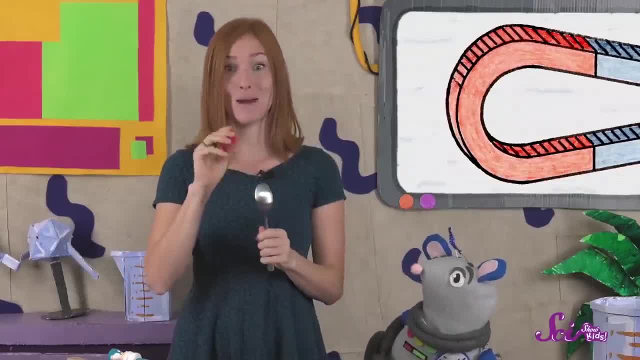 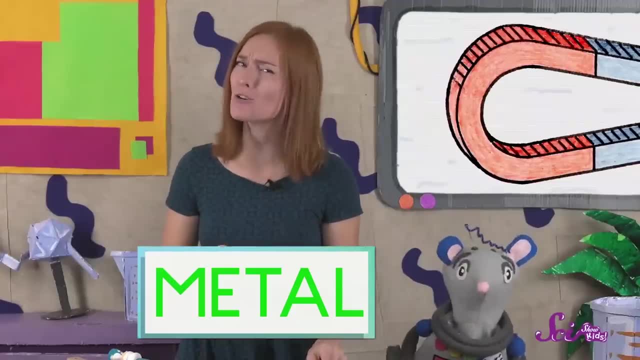 And there's something they all have in common, something that makes them similar enough to be attracted to my magnet. What do you think it is? Squeaks? You're right, They are all made of metal. Things that are made of metal are usually pretty shiny. 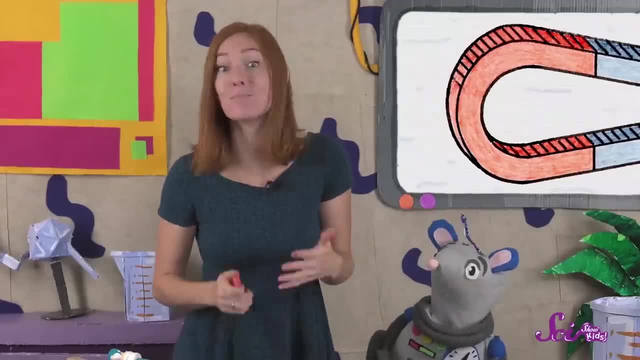 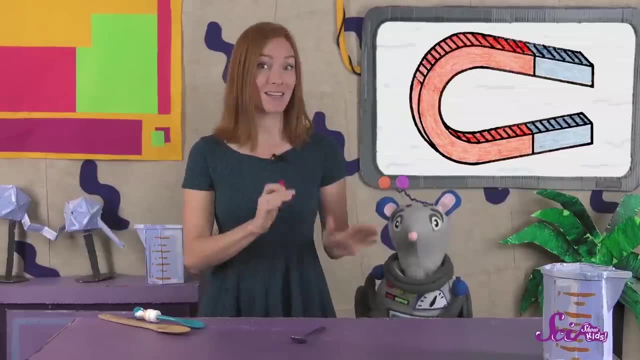 And they're often hard and kind of heavy for their size, Like how the metal spoon is heavier than the plastic spoon, even though they're around the same size. A magnet attracts things that have metal in them, but only certain kinds of metal. 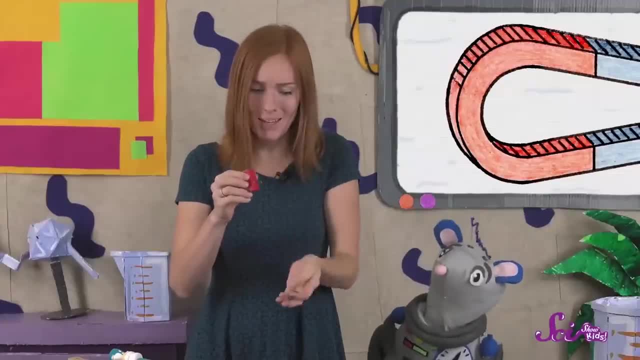 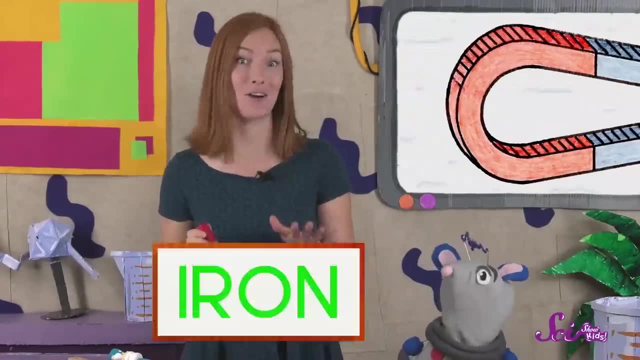 metal, not all kinds. Our magnet attracts this paper clip, but not this coin, even though they're both made of metal. One type of metal that is attracted to magnets is called iron. People use iron to make lots of different things, like fences and gates some kinds. 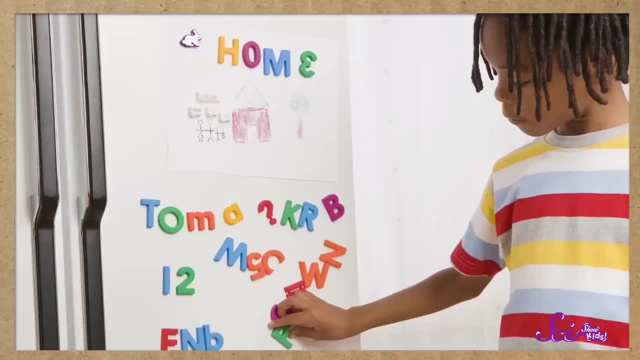 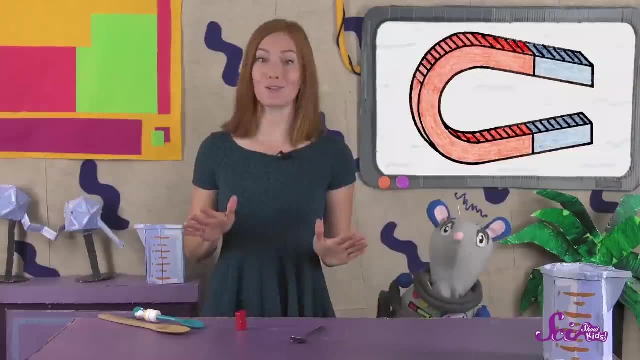 of pots and pans and lots of tools like nails and screws. And when a magnet sticks to a fridge, that's because there's iron inside the door. even though you can't see it, People use metals like iron to make something else too. 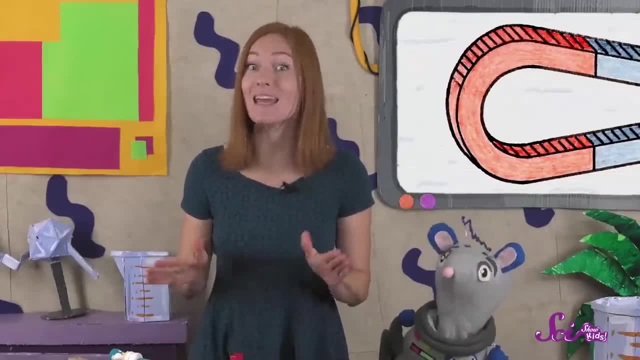 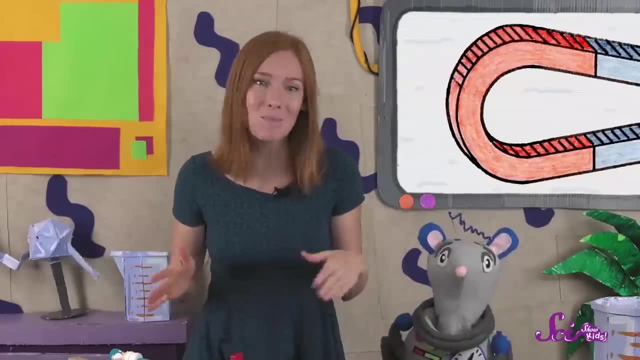 Iron is one of a group of special metals that people can make into magnets. Iron can do both: It can be a magnet and it can be attracted to a magnet. If you're curious about what other kinds of things are attracted to magnets, you can. 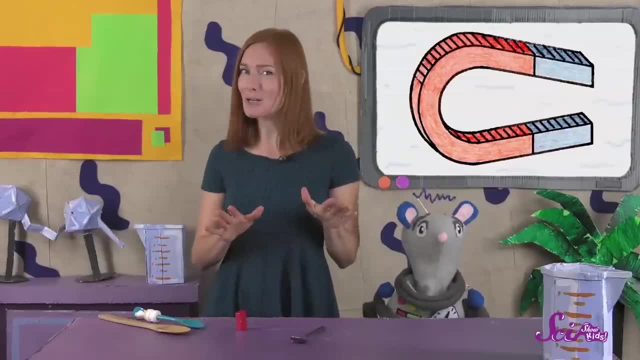 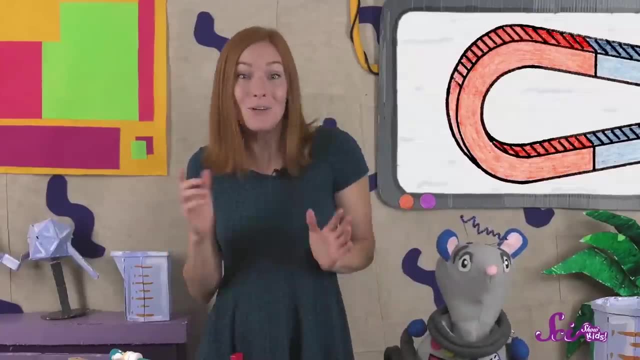 ask a grown-up to help you experiment. If you have a magnet, you can hold it up to different kinds of things and see if you can guess what the magnet will attract. Thanks for joining us. If you want to keep learning and having fun with Squeaks and me, hit the subscribe button. 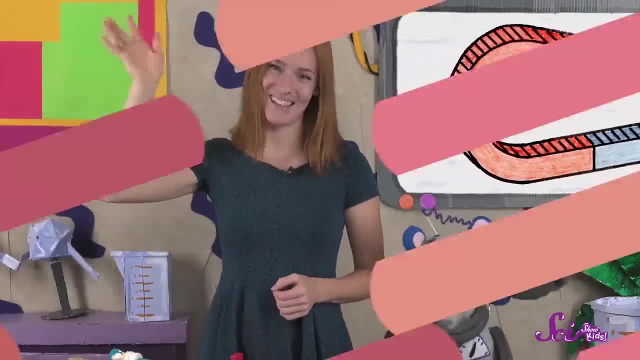 and we'll see you next time here at the Fort. Bye, Bye, Bye, Bye.